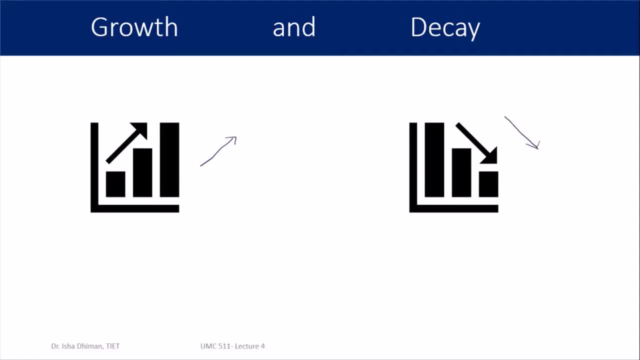 means something which is decreasing, which is falling, and usually, in most of the examples, we are looking at the growth and decay of certain physical quantities with respect to time, that what is happening to a particular thing with respect to time, either it is rising or it is decaying. So 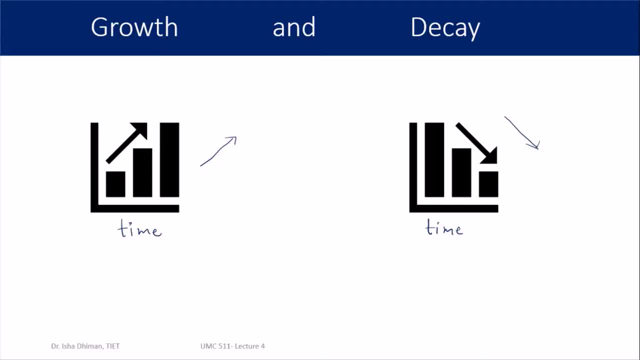 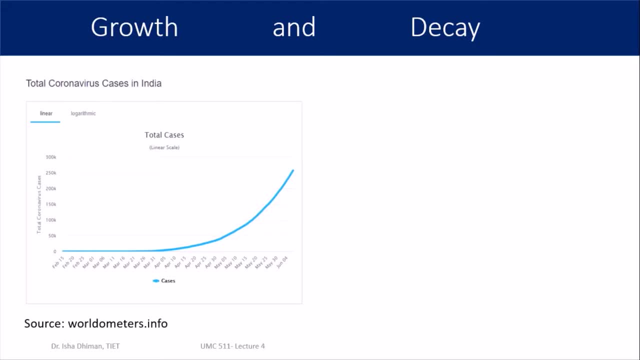 that's all about the meaning of growth and decay. and if you talk about the examples, then I could not find a better example. as you all are aware, with the current coronavirus global pandemic and this data has been taken And you can see that this is a total number of cases in India up to June 4. the data is 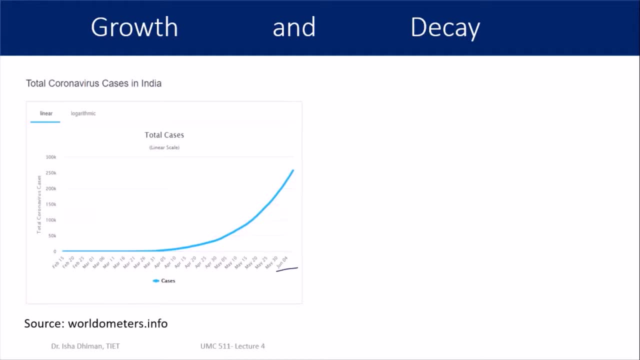 showing you that the number of cases is growing with respect to time. so obviously this side we are talking about time, so the total number of cases is on rhymes and if you want to have an example of decay, So here is an example in which I have shown that the death rate from air pollution per 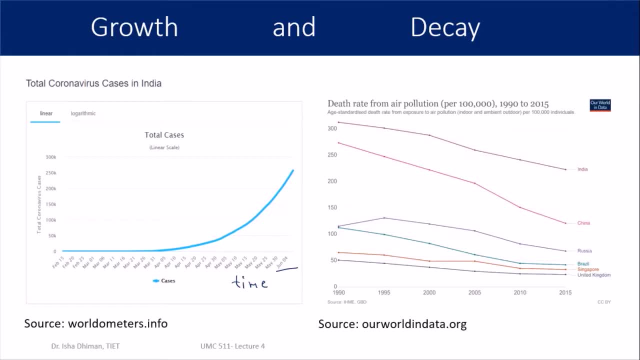 million 1990 to 2015. so this data has been plotted here for different different countries and if you look carefully at all the curves that you see a decay pattern. apart from this one, it first rises and then decays, but otherwise all these curves are actually depicting a decay with respect to time. so this is a 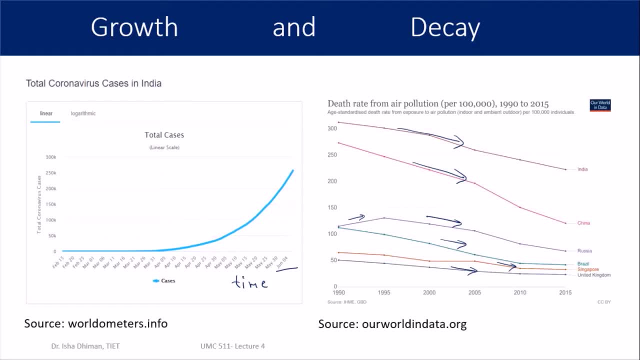 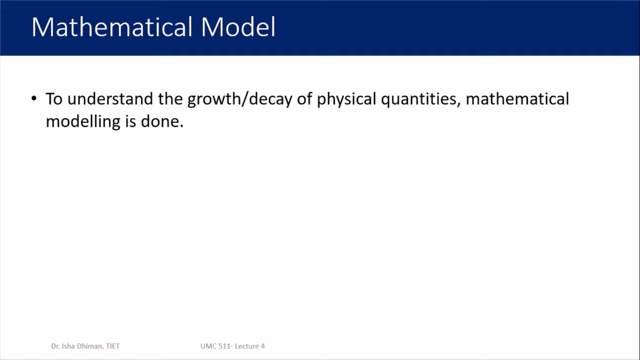 data based example that the data's are there coming from different sources. we plotted them and understood that we have the growth and decay. so now what is the next thing? the next thing is they want to mathematically understand them. we just don't want to look at the data and get the interpretation. the point is we 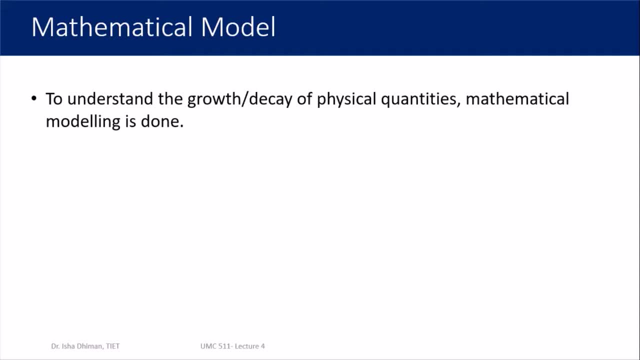 should be clear with okay, that something is growing or something is decaying, why this is happening. so, and if it is growing, how fast is the growth? how slow is the growth? how fast is the growth? how slow is the growth? how fast is the growth, or how fast or slow is the decay of particular quantity which we are? 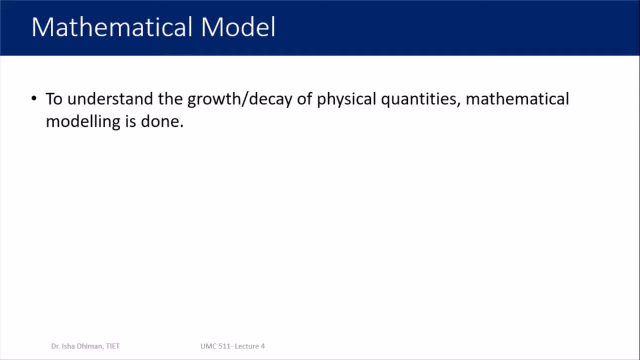 observing. so to understand all these questions and analyze that at what rate the growth and decay is happening, we want to have a proper mathematical model for the same. so that means the purpose of formulation of mathematical model is clear to us. we want to understand the processes happening in detail. what are 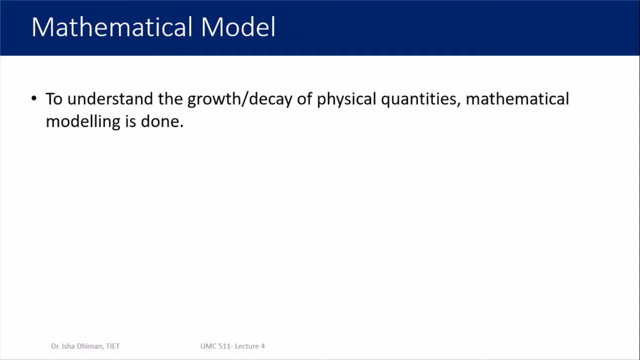 their reasons and what are their consequences. so for that we need mathematical model. so we identify that physical quantity which is changing with respect to time, either that is increasing or it is decreasing with time. so after identifying that physical quantity, we go towards the next step. for example, in this COVID-19 example, the physical 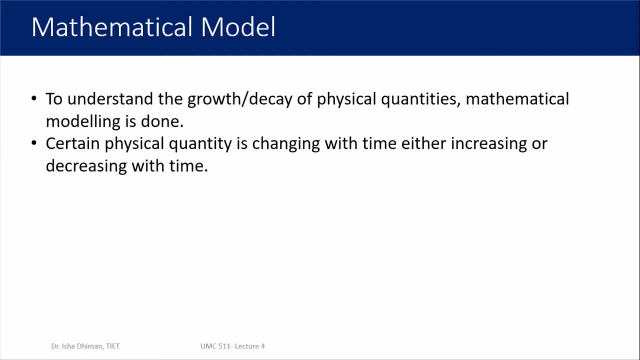 quantity is the number of persons, it can be the number of deaths, it can be the number of active cases, the number of recovered people, the number of quarantine people, so whatever is there which is measurable, so that one we want to understand how that number is changing with respect to time. so that's. 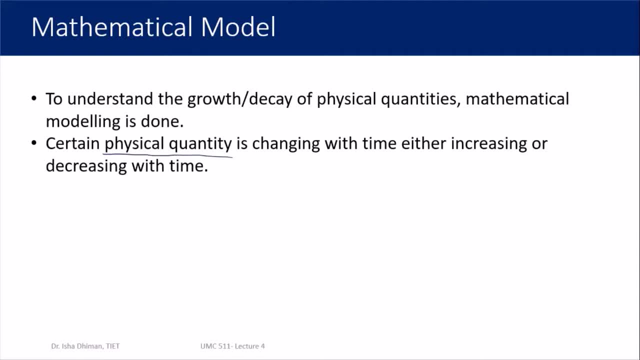 the meaning of identifying that physical, measurable quantity, whose change, whose temporal change, we want to understand. so, after identifying that physical quantity, the question arises: which type of mathematical model does our оh isıktان meglio عن physical quantity? which typeabei đây là attractions ter? 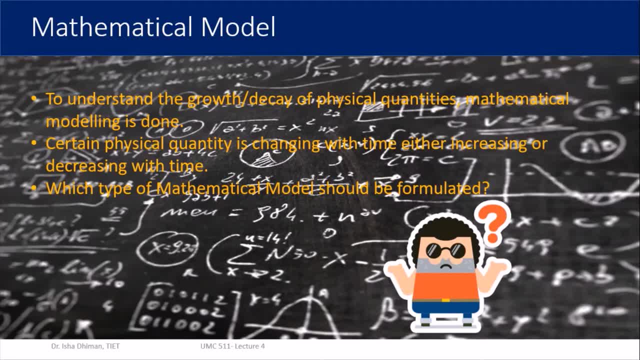 should be formulated As in the previous lectures I gave you the idea of that. they can be different kind of mathematical models. They can be linear equations, non-linear equations, algebraic equations, transcendental equations, system of equations or inequalities, theorems, differential. 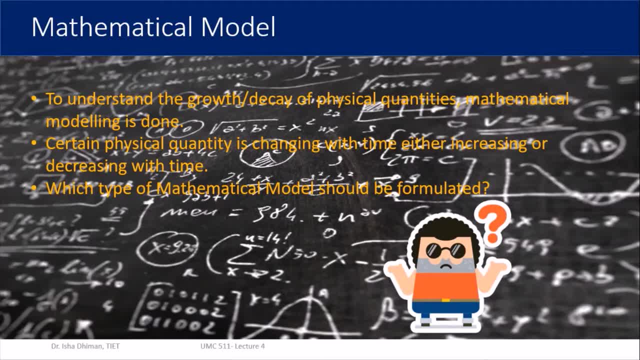 equations or integral equations. So these all are one or another kind of mathematical model. So now we are looking for an answer to this question. okay, that, okay, I have decided to model it mathematically, but what type of model I am going to formulate? So the answer lies in this famous 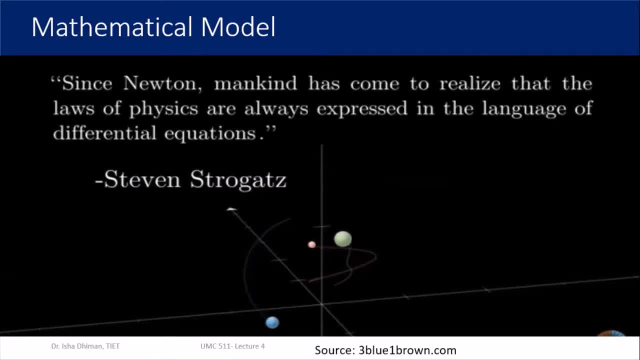 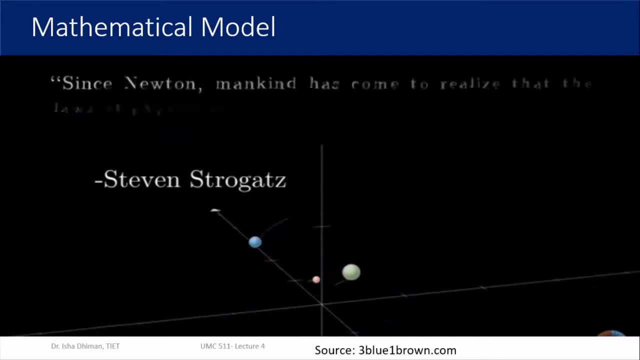 quote by Steven Strogatz. It says: since Newton, mankind has come to realize that the laws of physics are always expressed in the language of differential equations. So I hope with this quote it's clear that what kind of mathematically model we are going to talk about in this particular lecture. So let's move ahead. we have 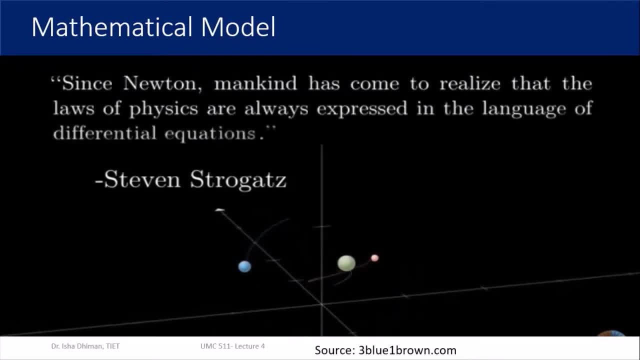 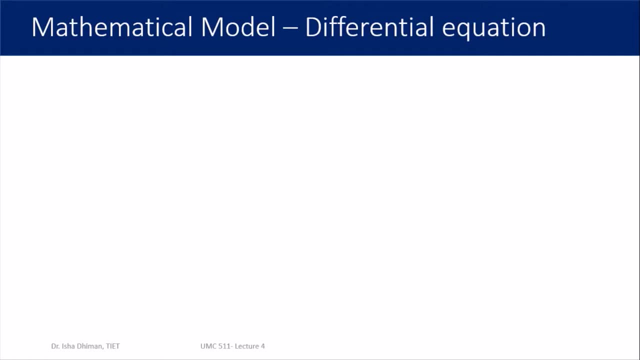 got the answer that we will be formulating a differential equation to understand growth and decay. So that's the answer. What is a differential equation? It's an equation that relates a function and its derivative. So there is a function which is depending upon something. So whenever we talk, 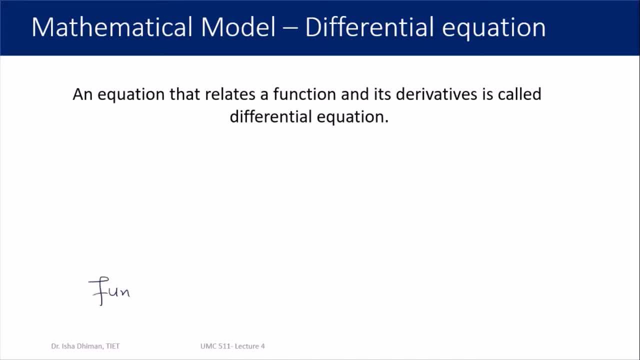 about function. so we mean this, the basic definition of function. I am not going to give you the exact definition, but just to recall you what is the function looks like f. so f is the some dependent quantity or the dependent variable. so it is the. 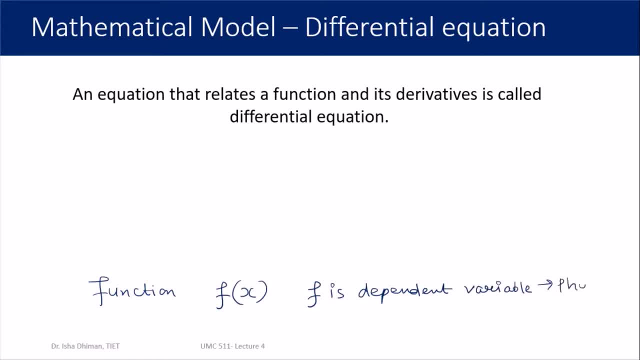 same thing which I was talking about. it is the underlying physical quantity and x is our so called independent variable. So whenever we talk about intermediate quantityN, So whenever we talk about broadly-dimensional strength, that means influences around a unit which we, whenever we talk about a function, there is some quantity which is depending upon other. 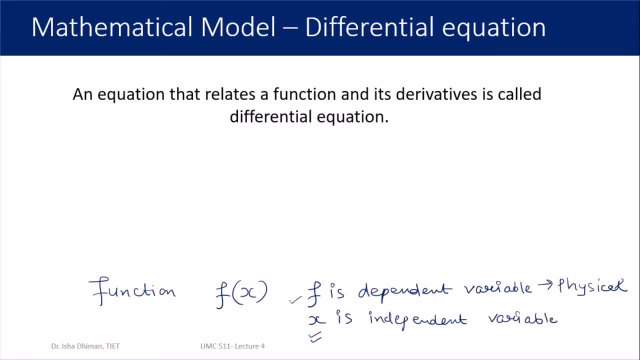 So if you change the independent variable, you get to see a change in the value of f. So that function involves it here and obviously the derivative. So why derivative is coming into picture? Because now you just recall what is the aim of this model. The aim of this model, 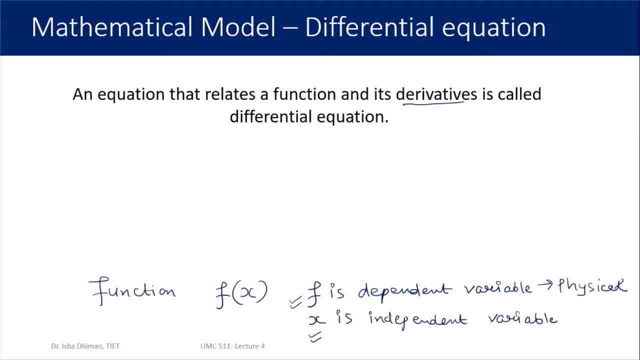 is to understand how the quantity is particularly changing with respect to time and if you recall from calculus that the meaning of derivative is the rate of change of the f with respect to x. So we know that f dash physically denote the rate of change of f with respect to x. So 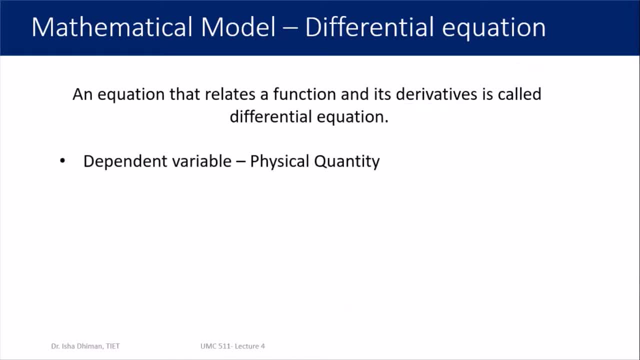 that's why derivatives are coming into picture. So these are the components of a differential equation. There is a dependent variable, which I have just told you: the physical quantity Independent variable. it's usually space and time, but today's lecture, most of the time, we are going to talk about the independent variable. So 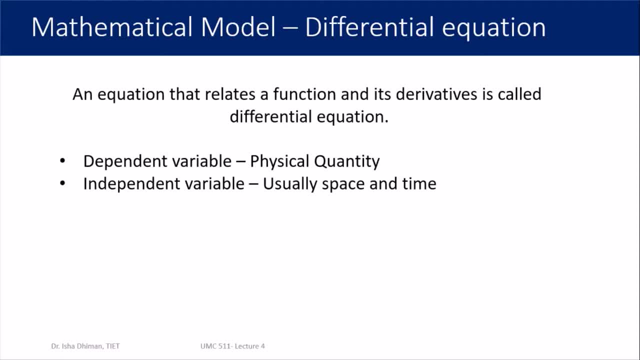 the time. we will be having time as the independent variable, because we want to understand the real world process which is happening in real time. So the changes we are observing are with respect to time. So our independent variable is going to be time, and then derivatives are involved. I have 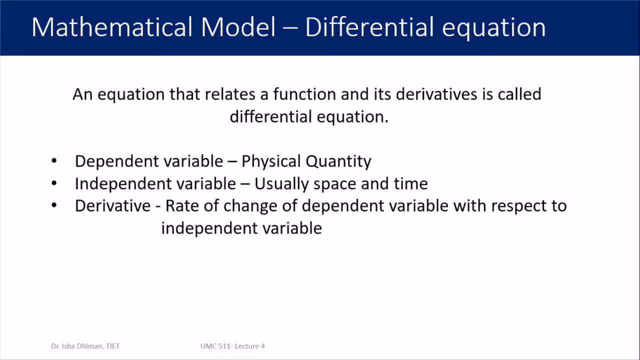 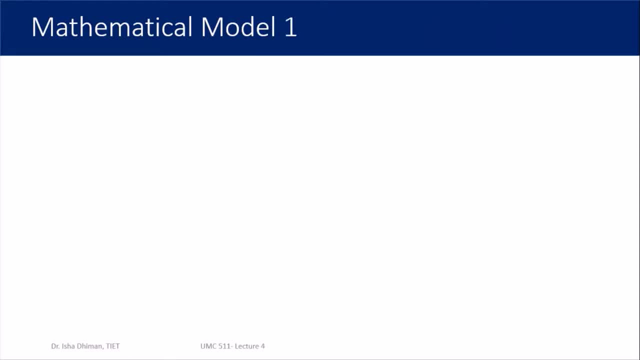 just explained you the meaning of it. The derivative is nothing but the rate of change of dependent variable with respect to the independent variable. So now let's start with our first model, Which I told you is going to be the simplest possible population growth model. So one thing I 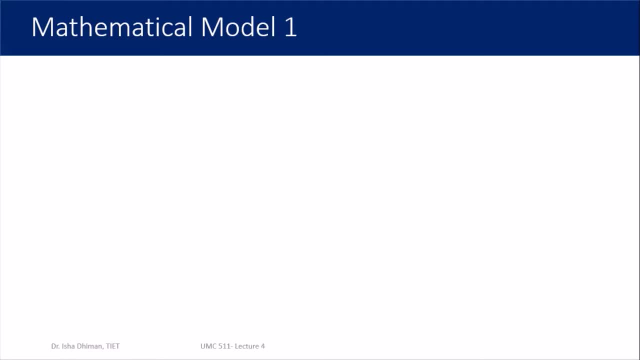 would like to make it clear here that, although the name I have given is population growth model, but it's not specifically. we'll be modeling the population growths, As I told you that the physical quantity can be anything. It can be the number of persons living in a particular area, how the 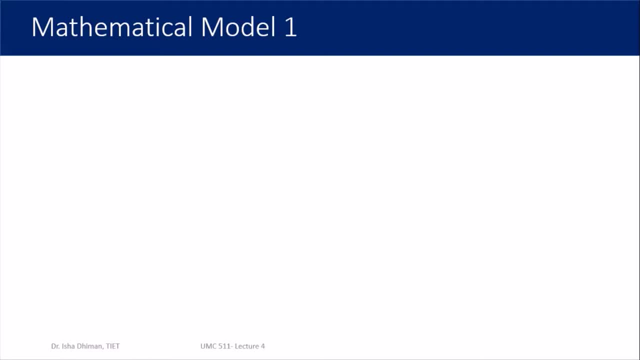 population of a country is increasing with respect to years. So that's also a way of looking at population growth and how the disease is spreading, how the infection is going to rise. So, although that number of infected persons does not literally mean the population, but still these models are called population growth model. So there, 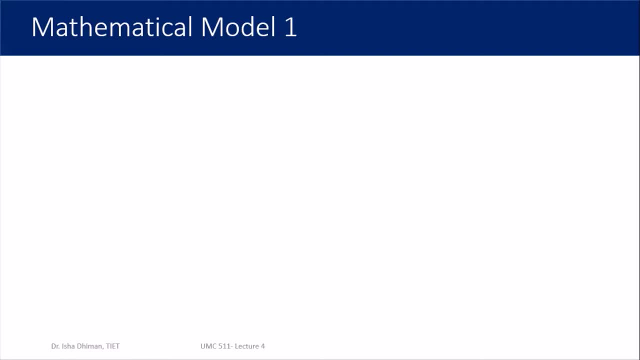 is a general name, population growth model. but it's not always necessary that the physical quantity is representing the population. So with that I'll give you the first example. So suppose you have a bank account and you deposit a fixed amount of money per month in your bank account. 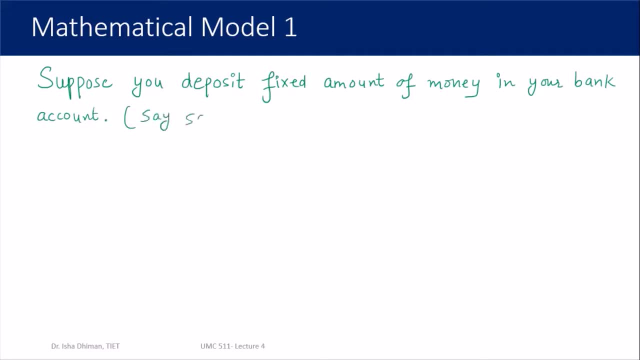 So you can take it like: suppose it's your salary which is deposited by your employer per month in your account. So since this is fixed number, so it is going to be a constant. So let this constant be denoted by K, K be the amount of money deposited in your account per month. so once you have figured, 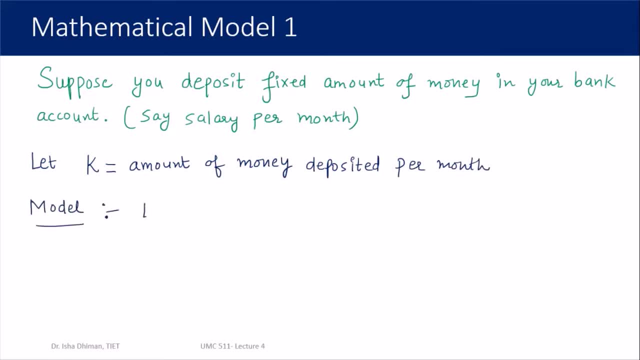 out that this is K, now I need to model it, and for model I need to define another variable that empty denote the amount of money in your bank account at any time. T because you start from some initial conditions and then why you are mathematically modeling this picture. 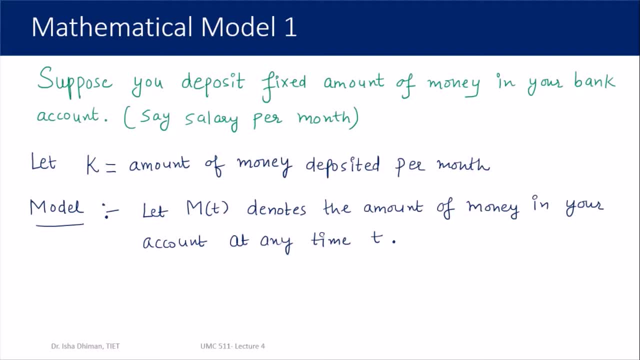 because you want to understand that. okay, if I have this much money deposited in my account every month, then at any particular time in future, I want to know how much money do I have? so I should have the formula for doing that. so, while deriving that formula for deriving, 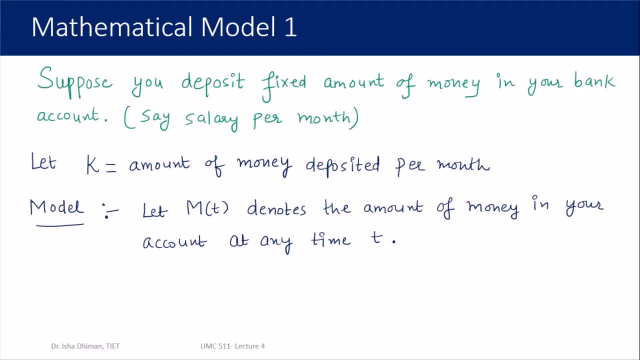 that formula. we are actually mathematically modeling it so you can say at this stage: okay, this is very easy, you don't need to actually formulate a differential equation for the same. but deliberately, I have taken a very simple example. So that's it, So that you can understand the basics of mathematical modeling. so I have defined my unknown, the. 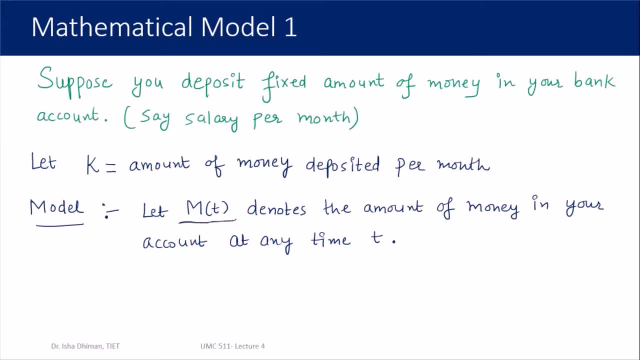 physical quantity or the dependent variable. it's clear that M is the dependent variable and T is my going to be the independent variable. so I just told you something which is changing with respect to another variable. so we need to bring into picture the derivative. so dM by dT. 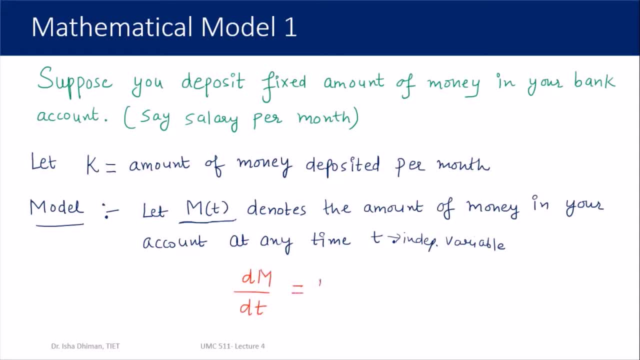 how M is changing. M is changing with respect to time is actually equal to K. it's a constant. because? why it's a constant? because it's stated in the beginning that you are depositing a fixed amount of money in your bank account and that does not change with time. that amount of money remains. 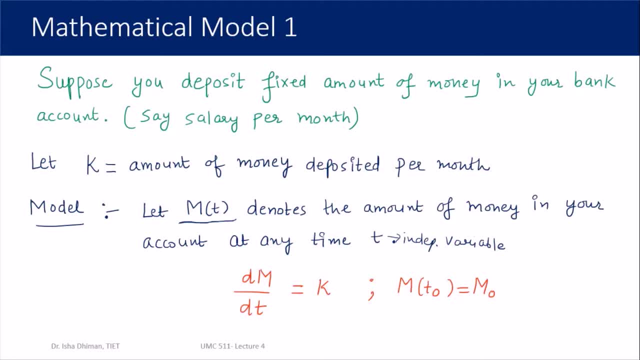 fixed, so the rate of change is constant. so that's why this is the model: dM by dT equals to K. and what is this? MT naught is equal to M naught. here, T naught is the initial time. Initial time can be zero also. for example, you start depositing it today, so today time. 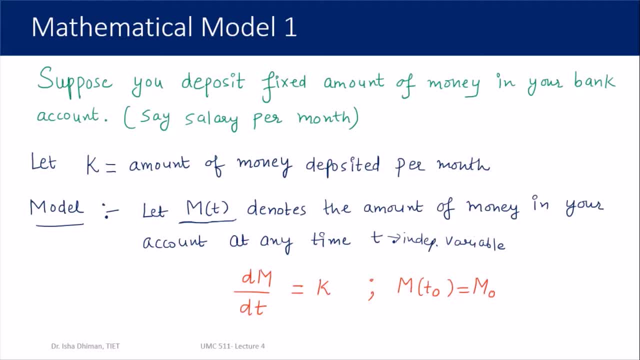 you can note explicitly or you can just refer this time to as zero time. so T naught is nothing but the initial time and M naught is the amount of money in your bank initially if you start from an account which is having initially zero money. so M naught will be zero in that. 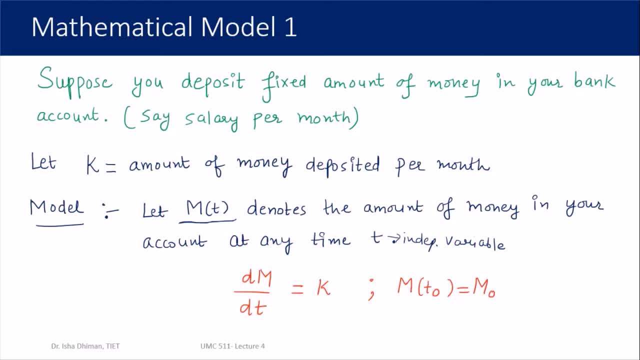 case. otherwise it will be having certain fixed value. So this is called a fixed value Initial condition. so this condition is very essential to find a solution of this differential equation, as you will see. So this problem is also called an initial value problem, although in general I am calling 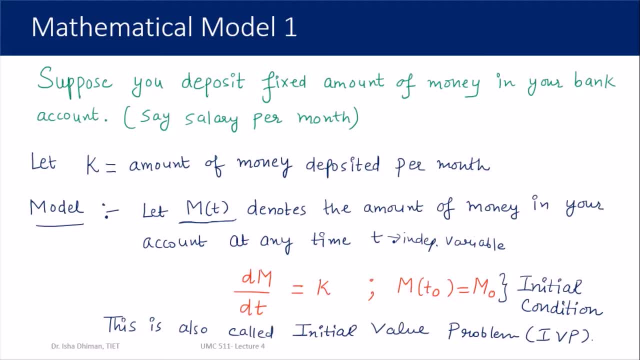 it a mathematical model, but specifically this kind of models in which you have a differential equation plus an initial condition given to us. we call it a initial value problem. So initial condition means you are always given the value, The value of your unknown. the capital M is your unknown, the value of unknown is given. 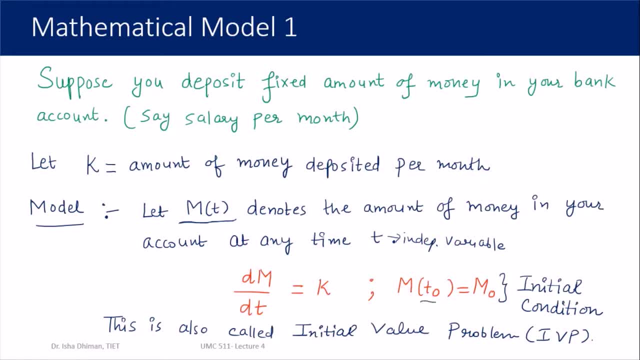 to you at a particular time, initial time. so initially you know the value and for rest of the future times you want to understand it that what is going to be the value. So these kind of problems are called initial value problems. So we are done with the model formulation. 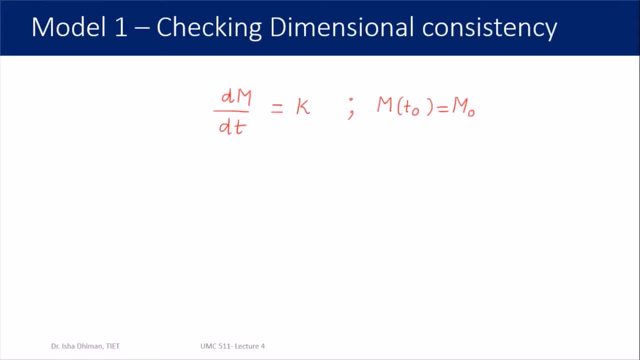 Now what is the next step? we need to check whether the model which we have formulated is dimensionally consistent or non-dimensional. So we are done with the model formulation. Now the next step is to check whether dimensionally consistent or non-dimensional. This is actual data. 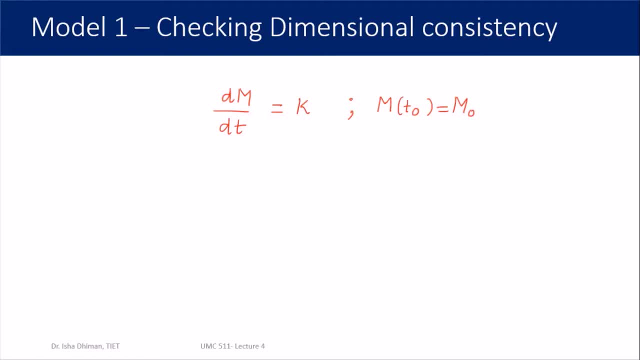 So how to check the machine that wecombine m by royalty, k is t minus 1, because k is money deposited per unit time. that unit of time is per month here, so the dimension is t minus 1. so you can see both of these are same. so therefore our model is: 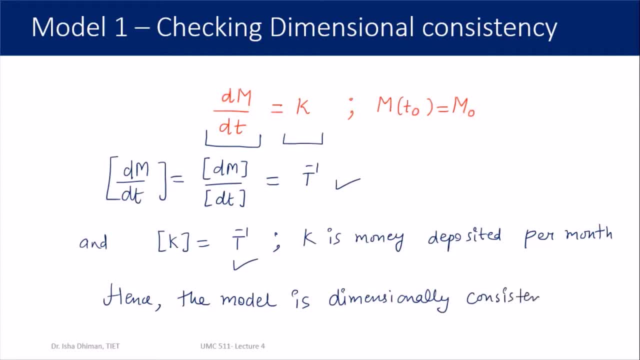 dimensionally consistent. so that's an essential step we need to do whenever we are formulating an model, a mathematical model, from the beginning, so once you are done with it, so now the next thing is we need to solve the model. if you recall the process of mathematical modeling it, we are 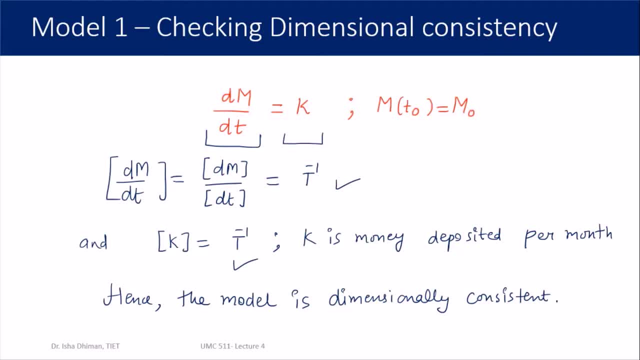 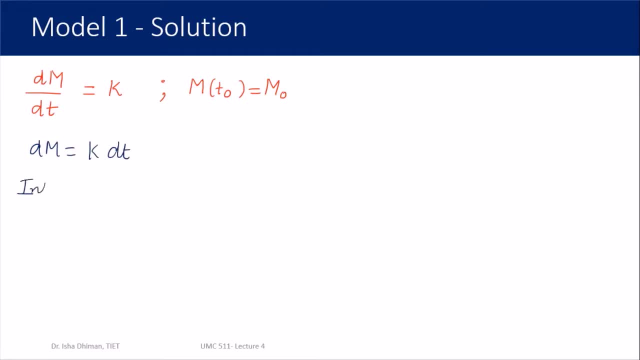 so dm is kdt if you integrate with respect to time on both the sides. so it's easy to see you're going to get. mt is kt plus c, where c is definitely the constant of integration. so never forget to add the constant of integration. so now how to find the value of constant of integration. so 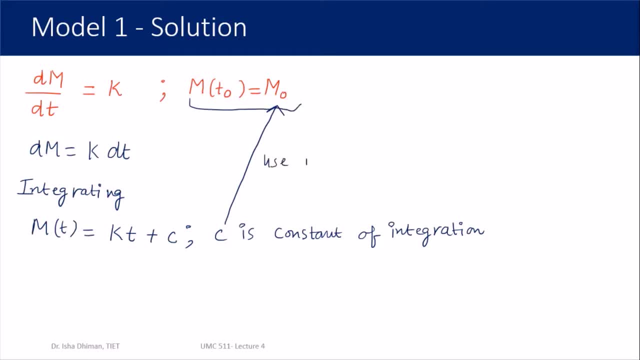 here we will be using our initial condition. so when you use this initial condition with specified values, you will get the value of constant of integration. so here we will be using the value of the value of your unknown at a particular time. so you will be using this to 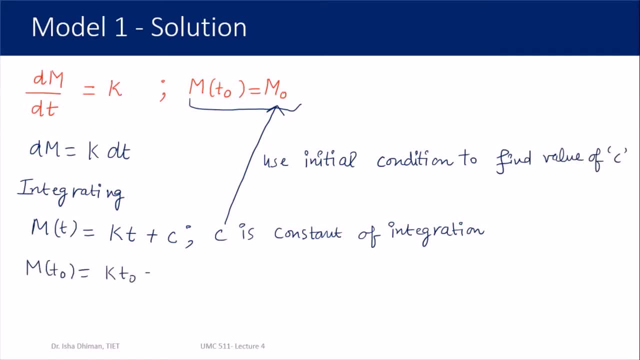 find the value of c. so m at t naught is kt naught plus c. this gives you c is equal to m at t naught minus kt naught, which is m naught minus kt naught. so by using the initial condition, we are able to. 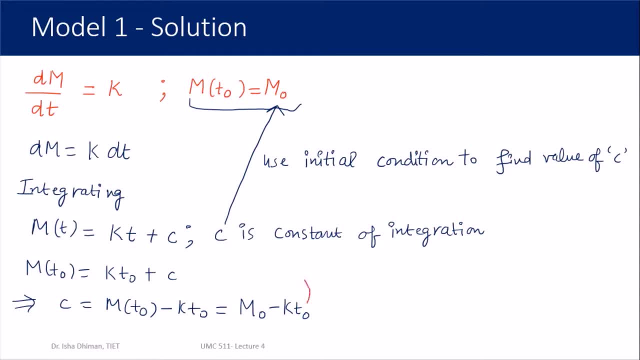 evaluate the value of c and now, once you have found what is the value of c, you substitute this value in the solution which we had obtained here. this was the solution: m at t is kt plus c. so this value of c you substitute here, you will get m at t is m naught plus kt minus t naught. so this is nothing but the solution of. 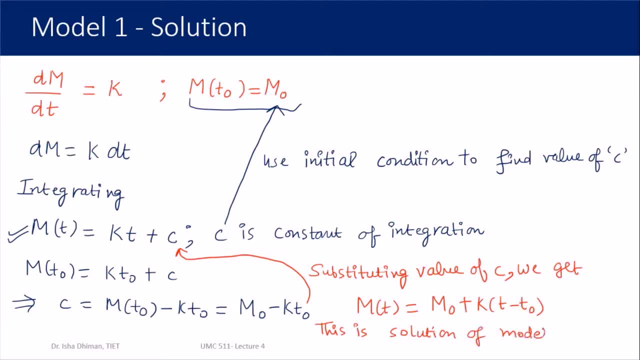 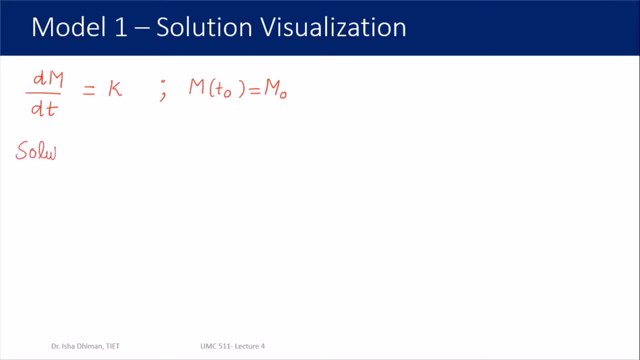 our mathematical model one. so that's how easy it was for this very simple problem. we formulated it and solved it. so what is the next thing in our mind? we want to now analyze this solution, that, what is the physical meaning of this solution, what this solution is telling us? so, basically, i want to visualize this solution. so for that, let's once. 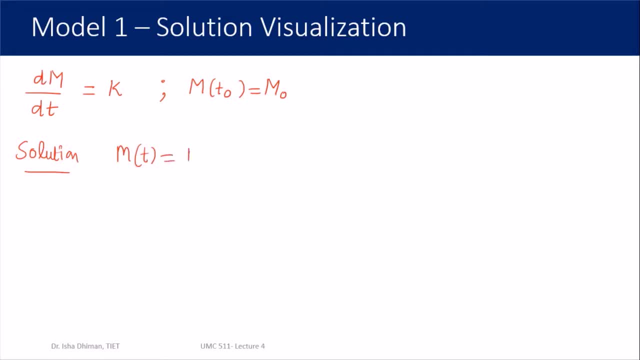 again write what is the solution which we have just obtained. this is m naught plus kt minus t naught. so in most of the cases our t naught is zero, because i even explained this you to earlier, that t naught is the initial time. so for simplicity you can write it as t naught plus kt minus t naught. 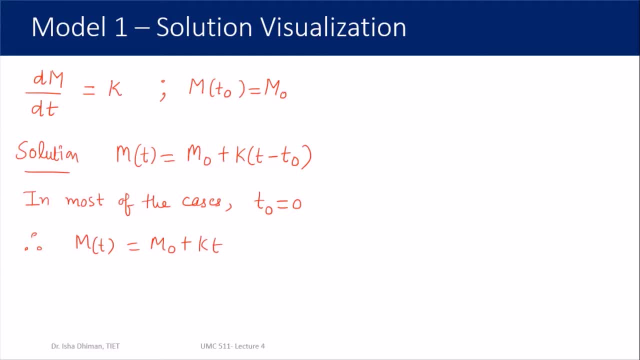 you can always take it- equals to zero, so this becomes the simple form of the solution. so m at t is m naught plus kt. so it's very easy to understand, because k is the amount of money which we are depositing per month. so suppose you want to calculate the money you have after six months. so it's the initial money. 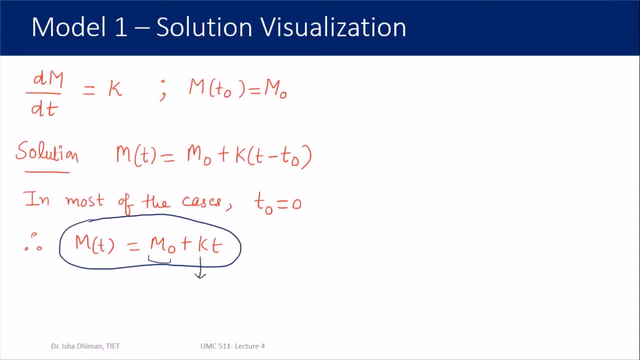 plus k, whatever was the amount deposited per month- say it was ten thousand dollars- into say t, t is six months, so it's some. initially suppose you started with, say ten dollars plus this. so whatever this turns out to be, that's your money at any given time. so that's obviously. we could even 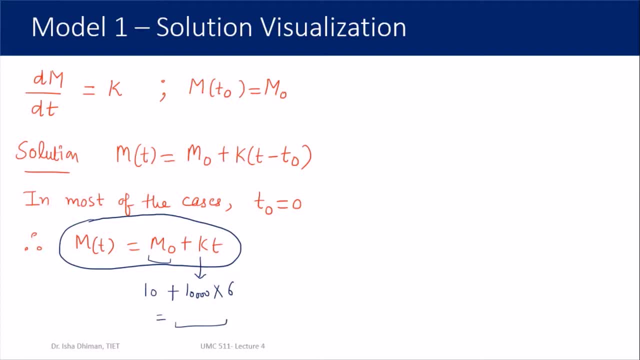 compute it without the mathematical formulation of the differential equation, but still the model is conceptually right. it is matching with the physical intuition we have for the solution. so what further i have done? i have given a specific value to m naught. m naught is equal to ten, which is giving me this. and this is nothing. but as you can see, i have plotted the solution for different values of k. 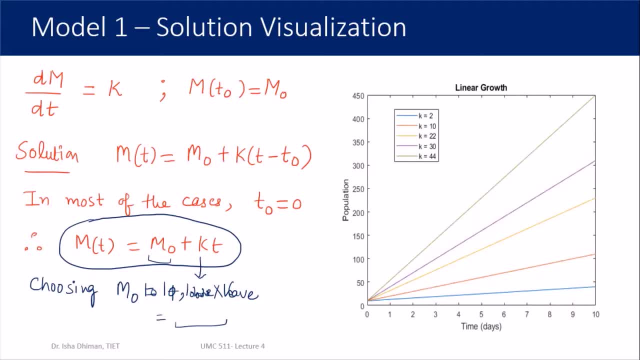 see. once you get the solution, it's very easy to identify your parameters. t is the independent variable, m is the dependent variable, while m, naught and k are my controlling parameters. controlling parameters means if i change the value of m, naught and k, i'll get a different solution every time. 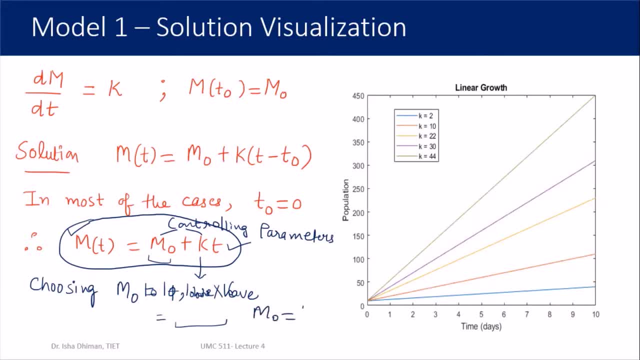 so i have fixed the value of m, naught equals to 10 here, and for different values of k, i have plotted the curves and all of you can see are straight lines, because even without plotting all of you we can understand that the solution is going to have a linear profile. so that's the reason. 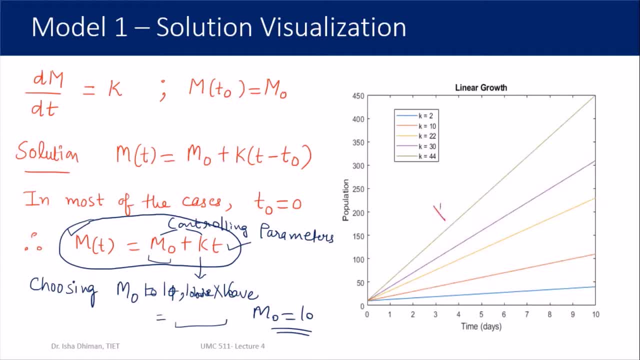 this is called a linear growth. and what is this k denoting? k is nothing but the slope of these lines. so because this is a linear growth as it is depicted from its solution curve, so that's why this model- dm by dt equals to k- is called a linear growth model. so whenever there is a quantity, 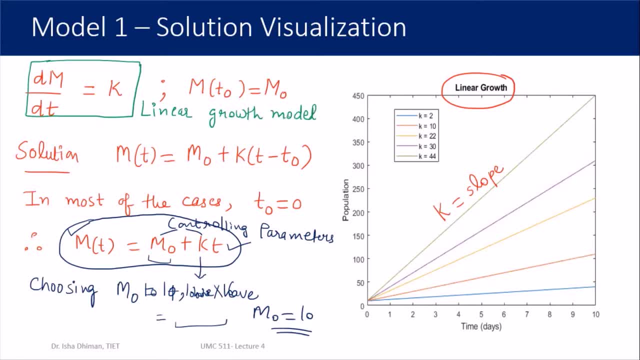 which is changing at a fixed rate with respect to time. so this is coming out to be linear only because k is independent of anything. k is just a fixed number. that's why it's turning out to be a linear growth model. so dm by dt is equal to k is a linear growth model. this is growth because k is. 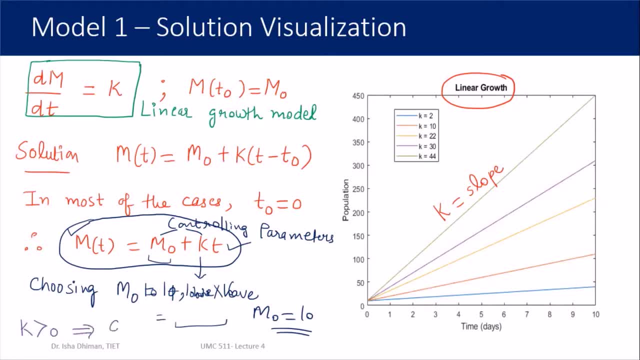 positive. so if k is positive, we call it a growth model. however, if k is negative, we'll be calling it a decay model. so the same model can act as a growth as well as decay model, depending upon the parameter k. right, so that's the visualization of the solution of model one. so now we want to be. 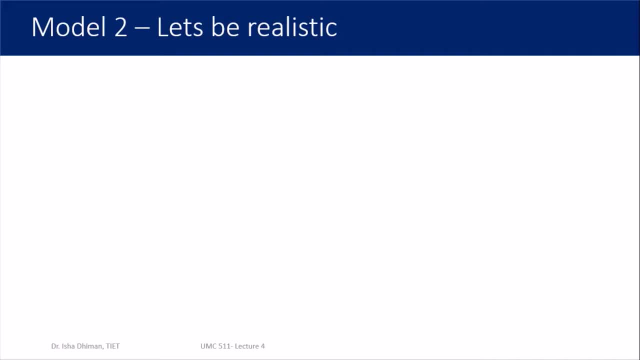 more realistic. so i want to move towards our next step, which is called generalization of model one, to something which is more appropriate, towards a reality. so, with this example, i want you to explain, with a very important step which usually is done while performing research in mathematical. 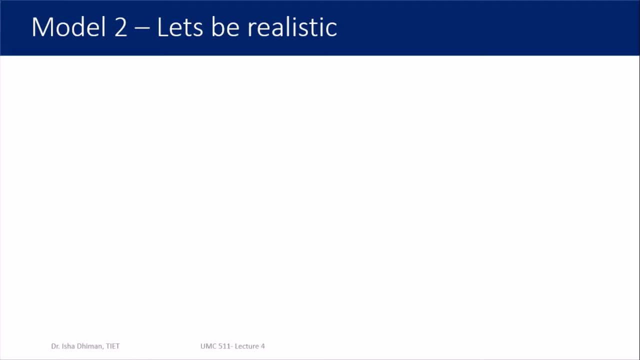 modeling. so whenever we want to construct a model of any real world phenomena, the first thing we have to do is that we just don't look at the construction of the model out of the black box. we just don't do it scratching from the base. we have to do it by looking at existing models. so you figure out. 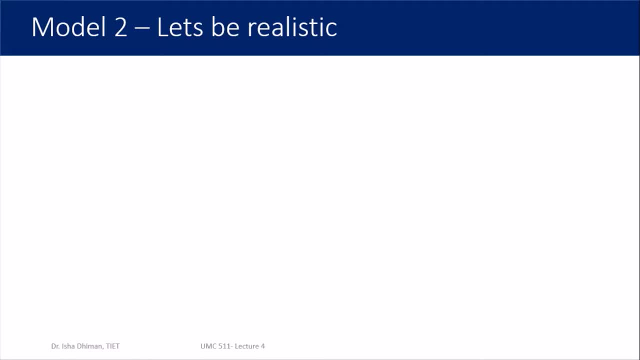 any existing model and then try to generalize it, try to point out a factor which was not involved in the previous model, and that will give you a more realistic model. so same technique i am going to use here, that to me, my model to be more realistic, i need to incorporate a factor which 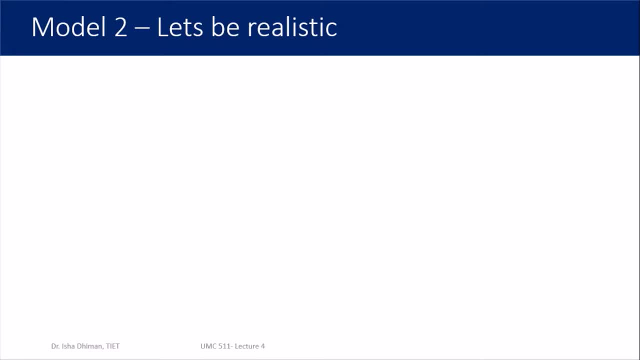 was not present in the model one. so model one was obviously a model of a real world phenomena. so we have to do it by looking at existing models while working on it. and this is all about that. the rate of money changing with respect to time in your bank account is fixed, so because you are depositing money every time, but in real life we do. 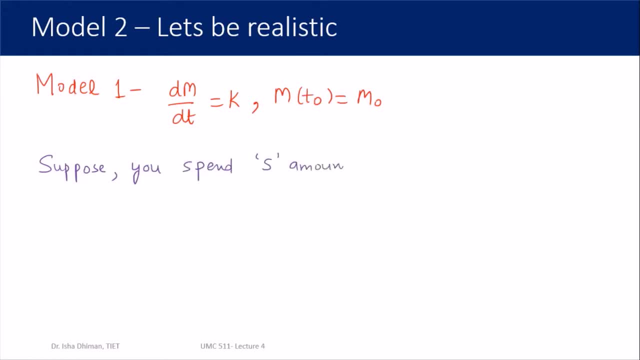 not only deposit money, we do spend as well. so here we have some amount of money you are spending per month and that is also fixed at s. so dm by dt turns out to be k minus s, because k is going to be going to be added, s is going to be subtracted because that your, that is, your spending from the. 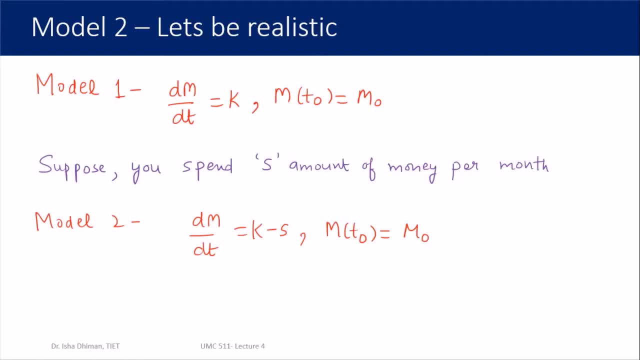 account. so, and that is also independent of time, so s also has to be taken to be a constant. but this model is definitely more realistic than model 1 because it is also incorporating spending and, moreover, this is called a generalization. model 2 is called a generalization of model 1. 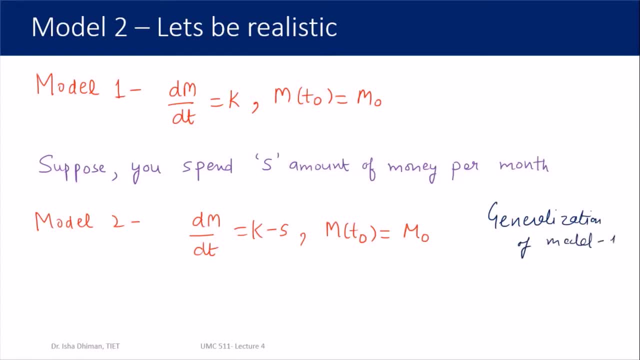 what is the meaning of this word generalization? that if i put s is equal to 0 in model 2, what i am going to get is model 1. so that means model 1 can be easily obtained from model 2 by changing or particularly fixing the value of certain parameters. so that kind of models are called the. 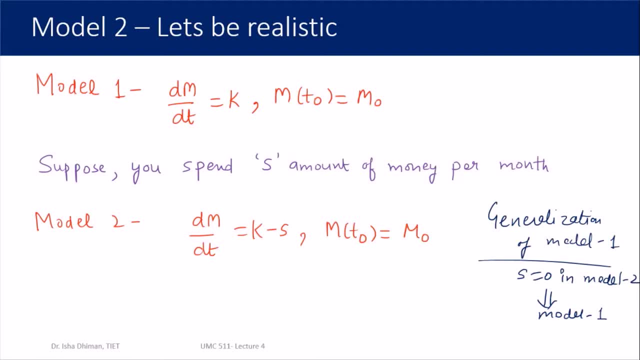 generalized models. so even if you study only model 2, then all the dynamics of model 1 can also be studied from the same. and if you talk about solution of model 2, so it's very easy to solve because on the similar lines you can solve it the way we have solved model 1. so it's just the differences instead of 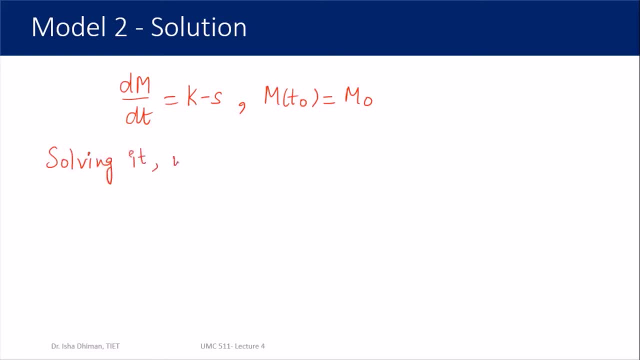 k. there is the term k minus s, so i'm solving it exactly on similar way. so i'm getting the final solution is m naught plus k minus s into t minus t naught, and again you can put the value of t naught equals to 0 for that. so that's how you solve it again. and if you talk about solution of 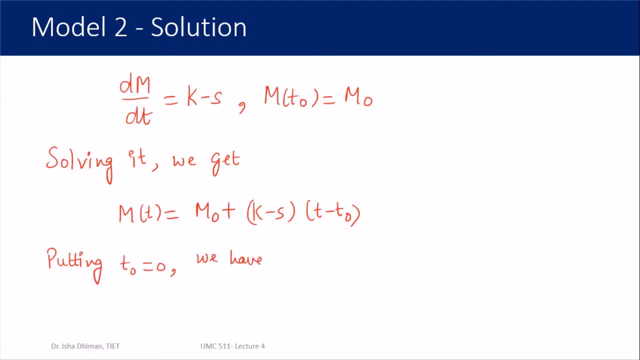 for simplicity. in that case we will be getting mt is equal to m, naught plus k minus s into t. so that's the solution of model 2. now we want to move towards the next step, that interpreting this solution in terms of real world. what this model is depicting, if you draw the graph of it, this is: 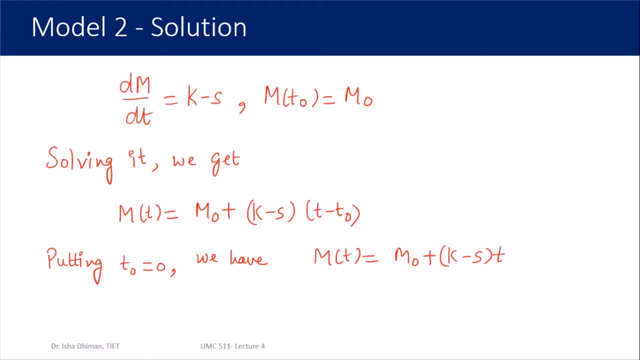 also coming out to be linear, but this time it is dependent upon the value of k and s. see, in the previous model, m, naught and k were the controlling parameters, but in this model there are three controlling parameters: m, naught, k and s. so let's try to analyze this solution in terms of the 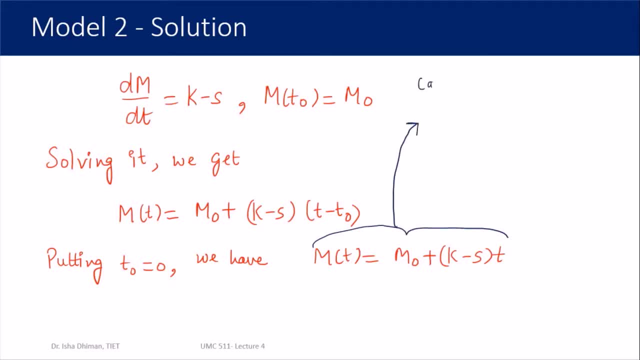 controlling parameters. suppose m naught is fixed. so case one is: when k is greater than s, that means you are earning more than you spend. in other words, you can say you are spending less than you earn. so eventually the amount of money in your bank is going to increase with time. 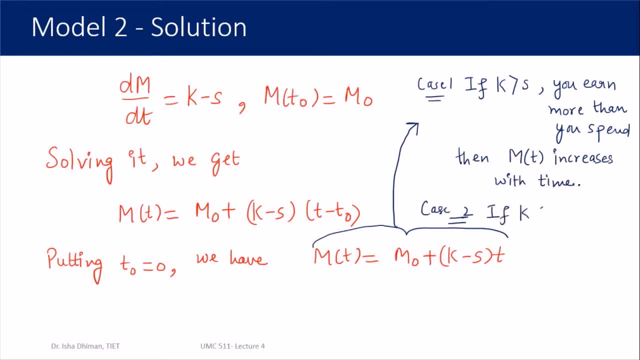 because the amount of money added is more but subtracted is less. but if k is less than s, then you are spending more than you earn. so in that case, obviously, what is going to happen? the amount of money in your bank eventually decreases dramatically with time and there will soon come a time when you will turn bankrupt. because- suppose initially- 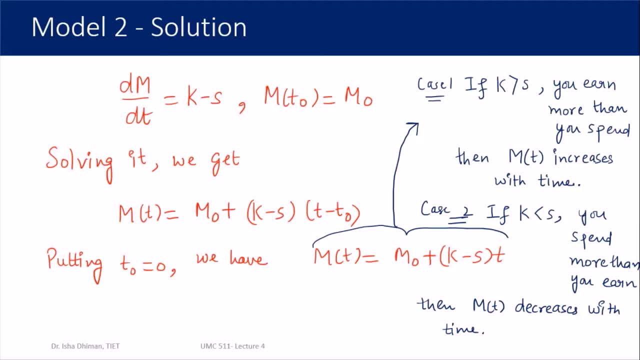 you had huge savings, but then later on, with every gradual month, your spending is going to increase as compared to your earnings, so you will eventually lose all the money you have. so this is the physical intuition of the model and it is actually matching with the reality. so the same information is coming mathematically from here, because if case one is happening, that 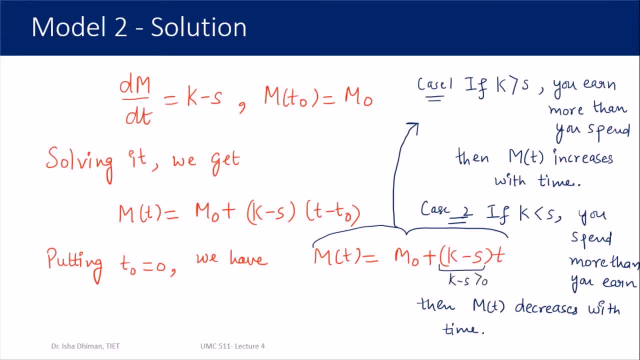 is if k minus s is positive. obviously time is something which is positive, so m naught the amount of money you started initially with plus something positive. that means m is going to increase. but if k is less than s, so in that case k minus s is negative. so by k minus s is negative. 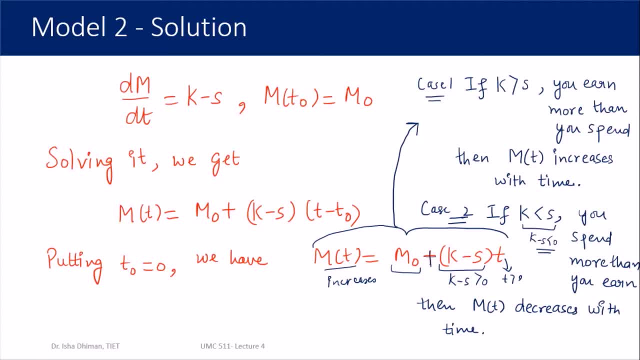 your m, you will lose all the money you have. so that is the physical intuition of the model and it is actually matching with the reality. mt is going to decrease with time. so that means our model solution is matching with the its physical intuitions. that's why this model is validated. this is correctly predicting what 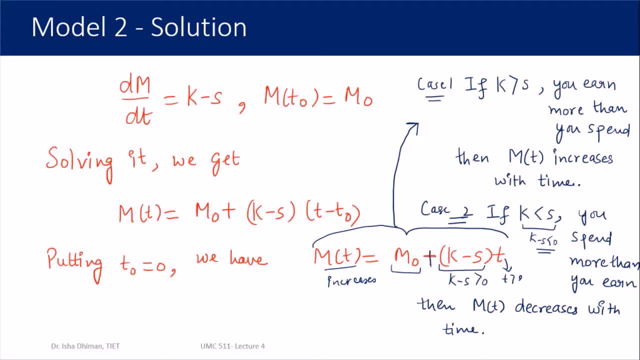 is supposed to happen. so here's a question for you. as i told you in the case 2, what is going to happen? that eventually you will turn bankrupt. so can you find the time taken by you in the case of k less than s in which you are turning bankrupt? so there's an exercise for you. you can. 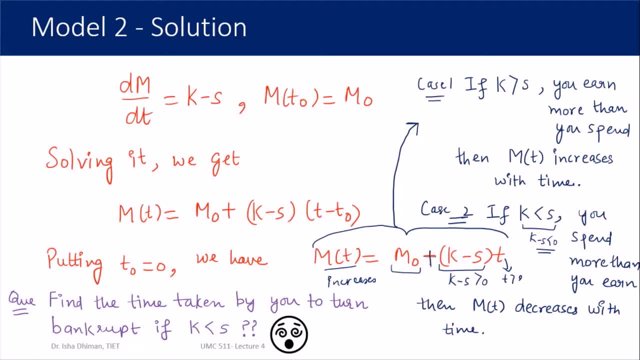 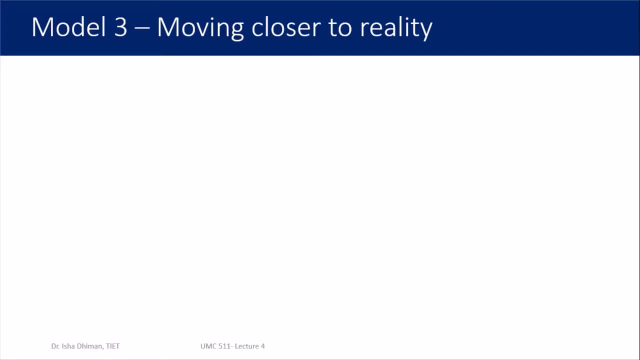 try. it's very easy. if you understand the meaning of the word bankrupt, so you very easily you'll be able to compute that. so that's an exercise. do that and get the answer okay. so the next thing is again one step more moving closer towards the reality. so this is one step more generalization. 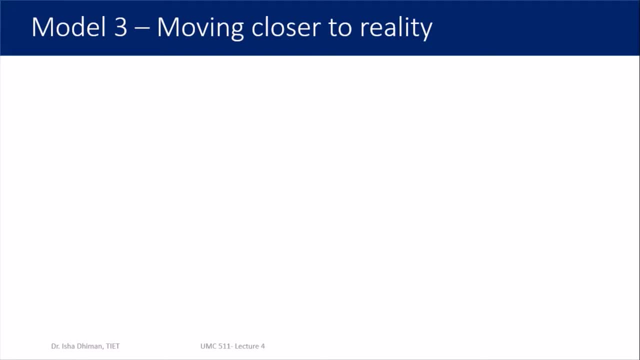 towards the real world process. so what's happening? in model 1 it was constant. in model 2, dm by dt was constant, minus spending was also there. but in model 3 i'm supposing it a bit more realistically that your spending is proportional to the amount of money you have in your account at that particular time. so that means 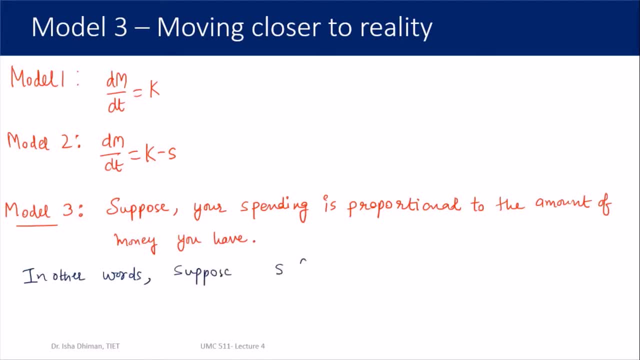 your s is not constant, while s is proportional to m. so mathematically it can be written as: s is a constant multiple of m. so say s is r into m. so this gives me dm by dt is k minus rm, and obviously with the initial condition m at t naught is m naught. so this is my model 3, so you can see that. 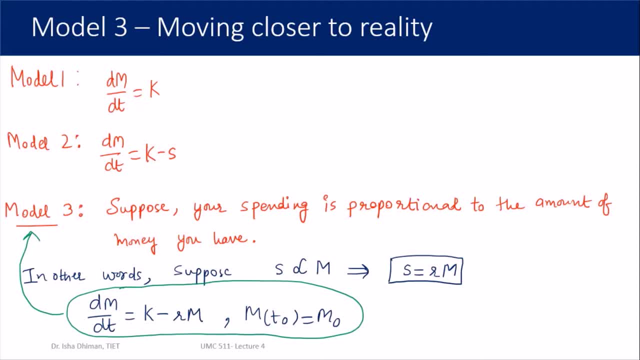 by imposing, or by assuming, another realistic assumption, that we do not just assume that we can spend every month a fixed amount. we spend according to the money we have. suppose initially you have less amount of money, so you will spend less, but as your savings are going to increase you will tend to spend more. so S is growing. 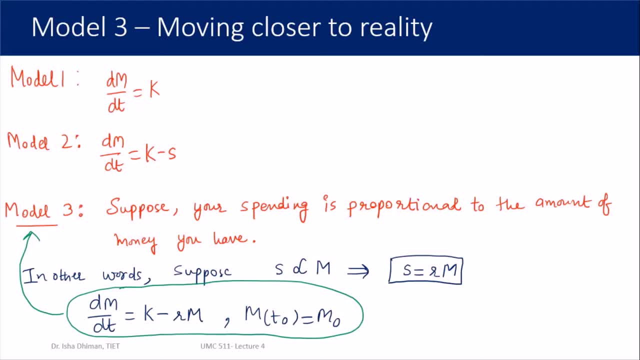 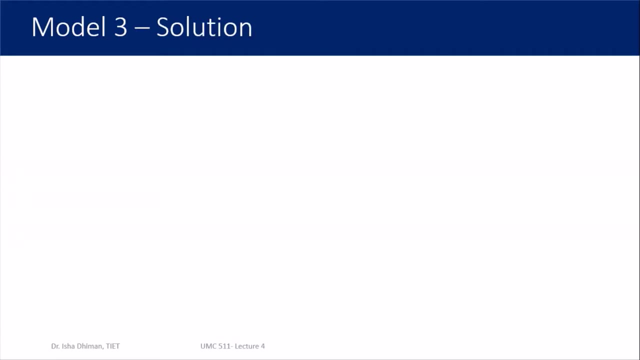 to be directly proportional to the amount of money you have. so this gives me this model. so clearly this is also a generalization of model 1, or you can also say model 2. so now we are interested in solution of this model. so here, because of the dependency of M in the right hand side, the solution 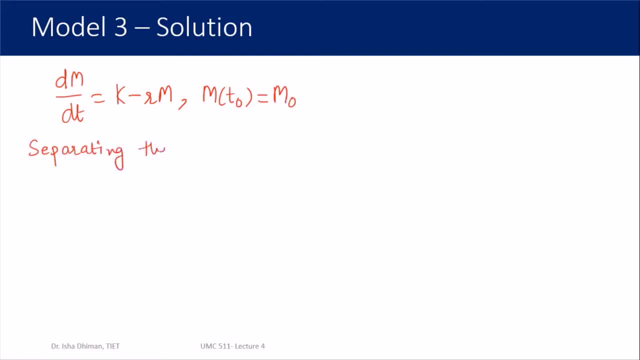 technique is going to be bit different. so I have used the separation of variables. so all of these techniques you have studied in your earlier classes and very easily you can figure out the solutions. so DM by K minus RM is DT, and then when you integrate both sides with respect to T, you get 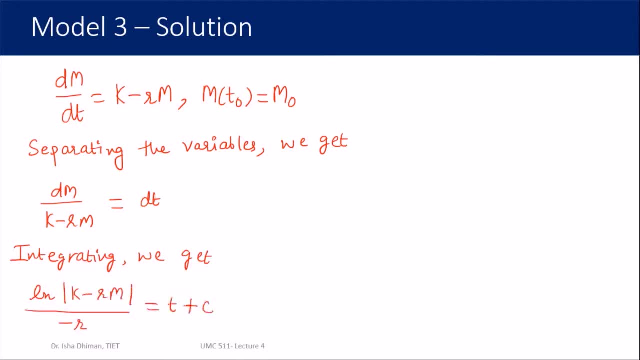 like this log: K minus RM by minus R is equal to T plus C. small C is the constant of integration. and then you just shift it to the other side. K minus RM is e raised to power minus RT into e raised to power minus RC. so this e raised to power minus RC, I'm 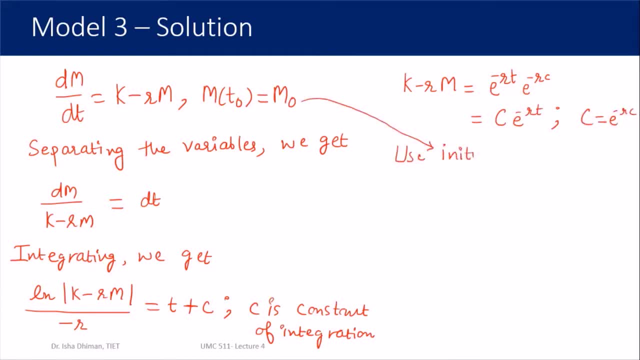 calling it capital C. so capital C will be found by using the initial condition. so when you substitute initial condition here you get capital C is K minus RM not into e minus e raised to power, RT not. and now you substitute the value of this capital C in the solution, you will eventually get your final solution in this form and T. 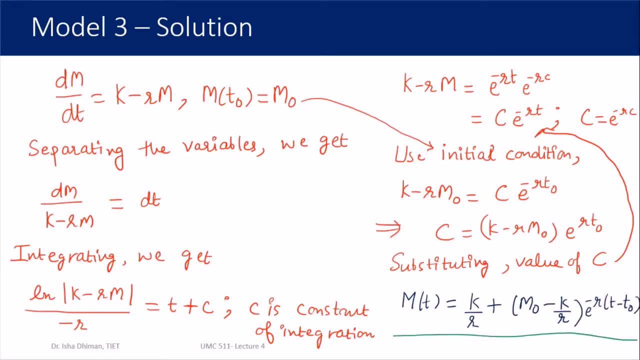 is K by R plus M naught, minus K by R into e, raised to power: minus R, T, minus T not. so this is not going to be difficult. you can do that substitution step and very easily you will be reaching this stage. so that's how the solution looks. 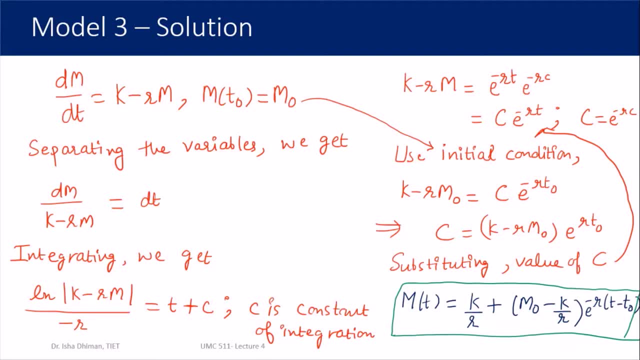 like. so it's no more going to be a linear growth model one and model two. both of them were linear. but model three is not a linear profile solution. its profile is going to be either exponential growth or exponential decay. so in what cases it is going to be decay or growth, that we have to see. but that 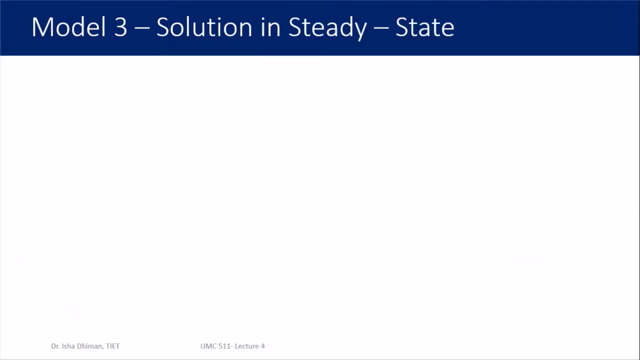 is the solution we are obtaining here. so now I want to give you another interpretation of the solution: that, instead of the solution directly, this alternate way of understanding the solution, which is called looking at the steady state of the system. so what is meaning of steady state? a dynamical system is said to be in steady state if there is no further. 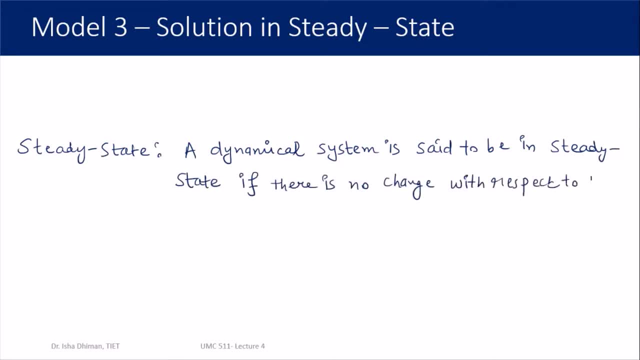 change with respect to time. so that means your system has reached a particular stage when the things have stopped changing with respect to time. so mathematically it means that the underlying physical quantity is derivative with respect to time is going to be zero. because if something which is 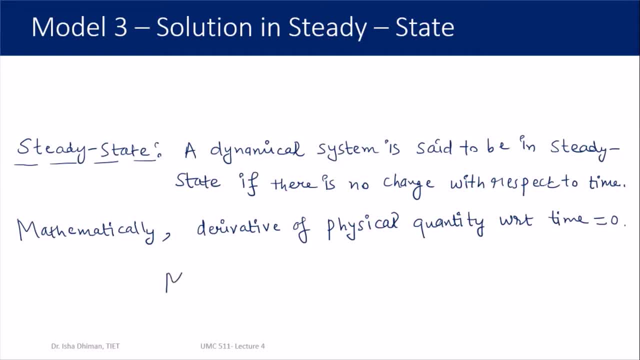 constant. so say your quantity is M. now it does not say depend on T. so in that case it means that B, M by D, T is going to be zero. so that state physically represent steady state and it's very important to look at the situation of the system. so that's why it is important to look at the situation of the system. so that's why it is important to look at the. 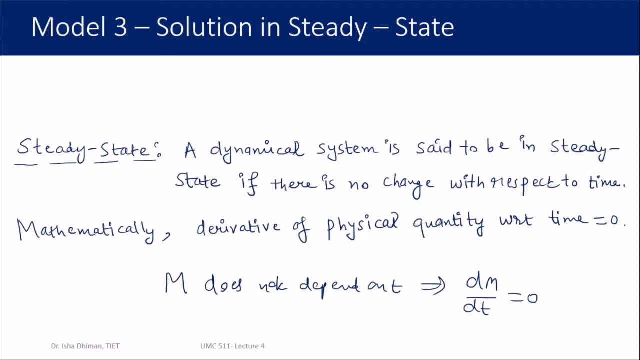 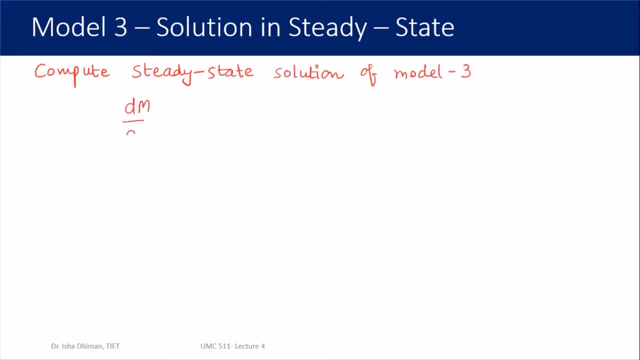 steady state because most of the times, very important and useful information is coming from the looking at steady state solution profiles. so let's obtain the steady state solution for this model three. we have already computed the general solution, but now I want to know you that how to compute the steady state. 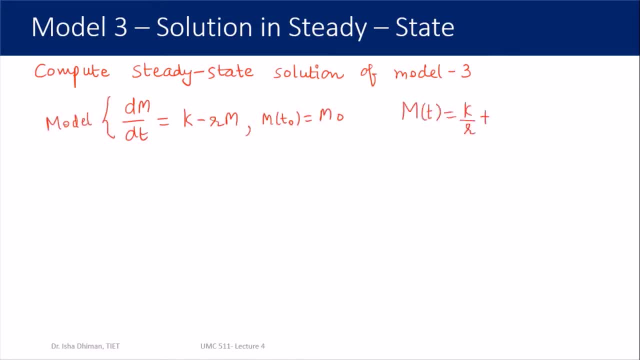 solution. so this is the model and this one is a solution which we have just obtained. so I will tell you there are two ways of obtaining the steady state: one from the directly, the model, and one from the solution. so with both the ways, I'll be computing the steady state, so directly. 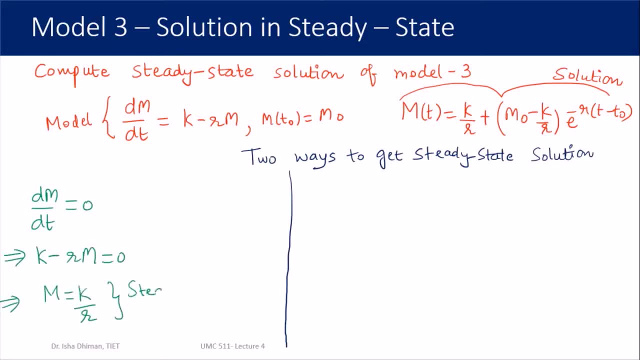 from the model you put just D, M by D, T equals to 0. this gives you M equals to K by R and otherwise from the solution if you want to get it. so as time approaches infinity, this factor e, raised to power minus R, T, minus T, naught, goes to 0. this again gives 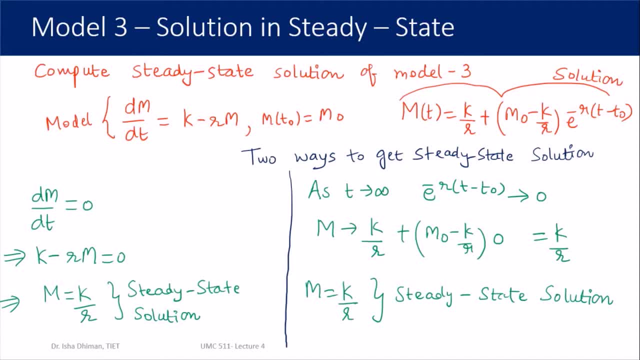 you M equals to K by R. so I can explain it again here. so the left-hand side has been obtained from the model. when you put D, M by D, T equals to 0. this gives me K minus R. M equals to 0. this gives me M equals to K by R. so this is the amount of. 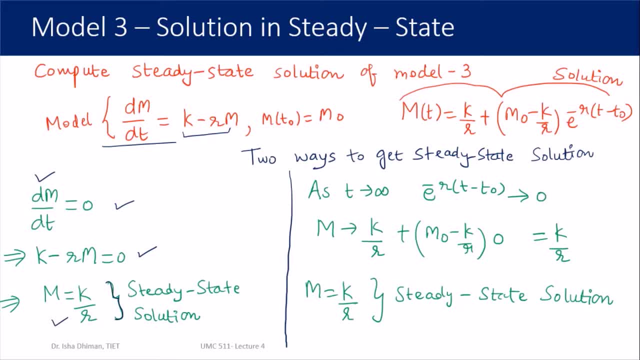 money I'll be having eventually after a very, very long time, because then things won't change further with respect to time. so this is a steady state solution and on this side, another way of obtaining steady state solution is from the solution. this is a solution which is giving me M as a function of T, but after a very, very long time, that means as T approaches. 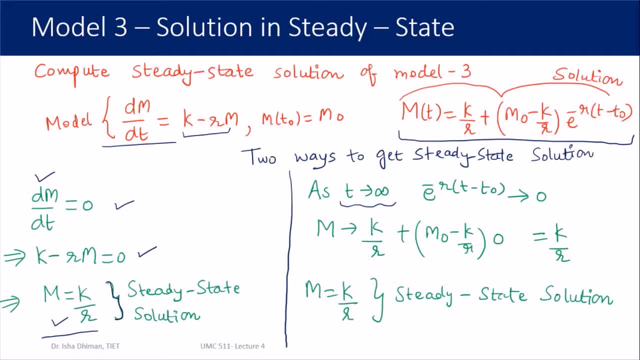 infinity. so you remember this technique: whenever somebody asks you to get a steady state solution from the solution, then you put T going to infinity. so whatever you will be getting is the steady state answer. so when T goes to infinity- e raised to power minus R, T minus- 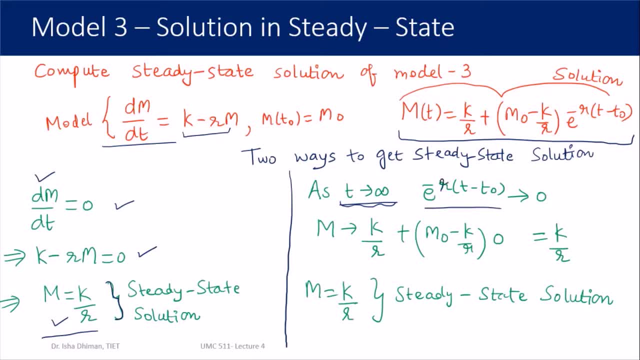 T naught goes to 0.. Why that is so? because R is something positive and obviously T minus T naught is also positive. so this quantity will go to 0, and if this will go to 0, so M will be just K by R. so you: 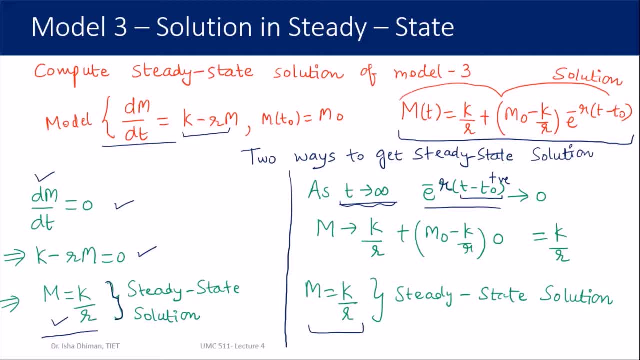 can see. obviously, the steady state solution is same. either you obtained it from the model or you obtained it from the solution. so that's how easy it is to obtain the steady state solution without even solving the model. I can directly obtain it from the differential equation. 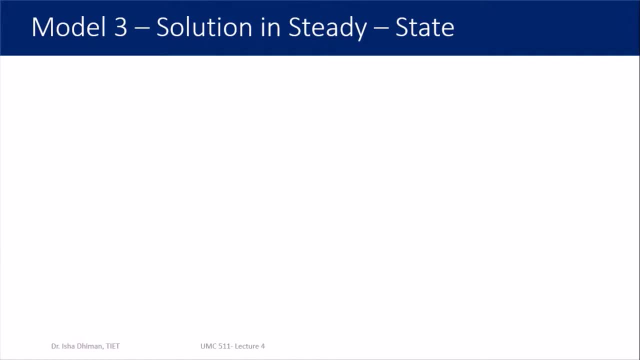 As well. so now let's interpret this. the solution which we obtained as steady state solution. M equals to K by R. we want to analyze this, that what is the meaning of this, or what is the consequence of this? so this is, as I've just told you, the amount of money in your 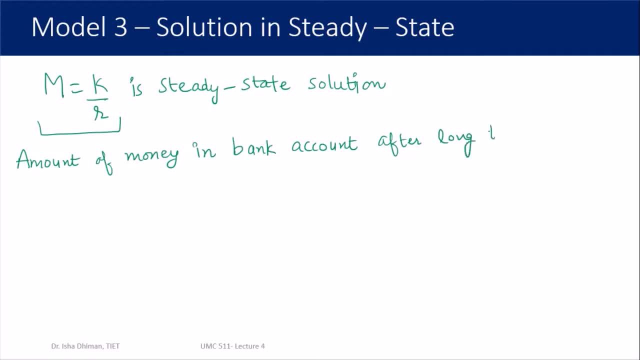 bank account after a long time. so that long time really depends upon model to model how much time it takes to reach it. So let's say you have a steady state, but in general this means this: so suppose M naught was a initial money. so this K by R is your final money which is going to sustain in the 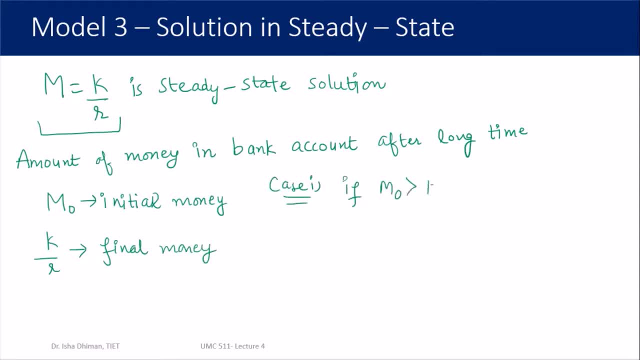 last. so case 1 is: if your M naught is greater than K by R means initially you had more money. so that means money is decreasing with respect to time because initially you had more money. and case 2 is: if M naught is less than K by R, that means money is increasing with respect. 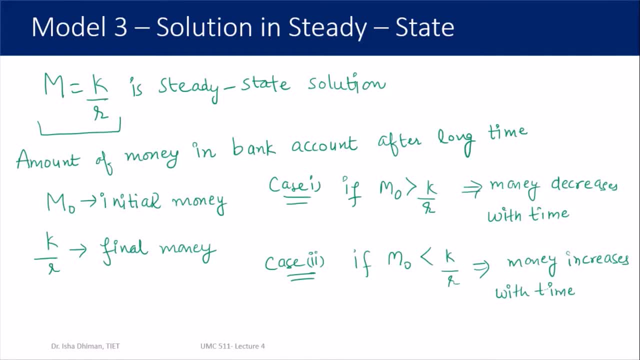 to time. So that means these controlling parameters are going to decide. you see how beautifully the mathematics is giving you the answer, because here K, R and M naught. these are your controlling parameters. so you can see how these controlling parameters, relations, are going to tell you. 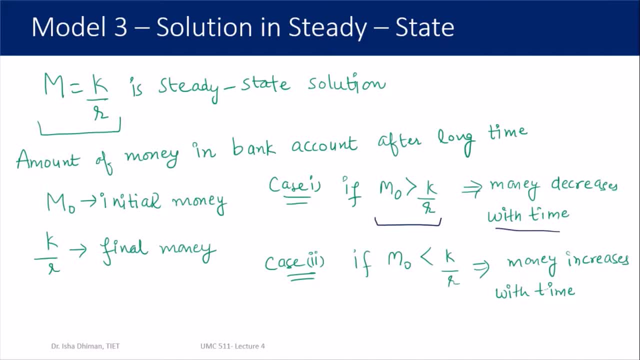 what's going to happen. so if you started initially with the amount and K and R, K is your spending sorry, K is your earning, R is a spending proportion. So if that ratio you are able to retain greater than sorry, less than initial money, in that case 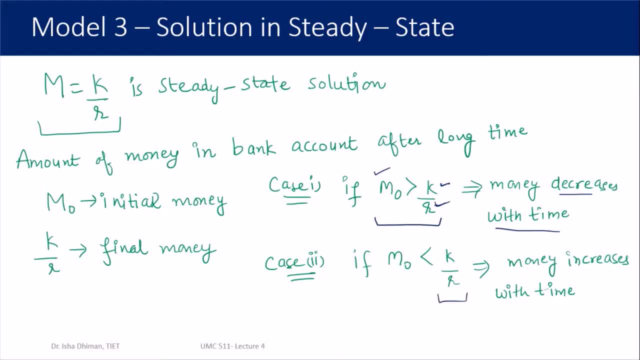 you are going to lose money. but if you maintain that ratio, greater than the amount of money you initially had, then your money is eventually increasing with respect to time. so by controlling your ratio of spending to earning, you can actually control the amount of money which you are going to have in future. 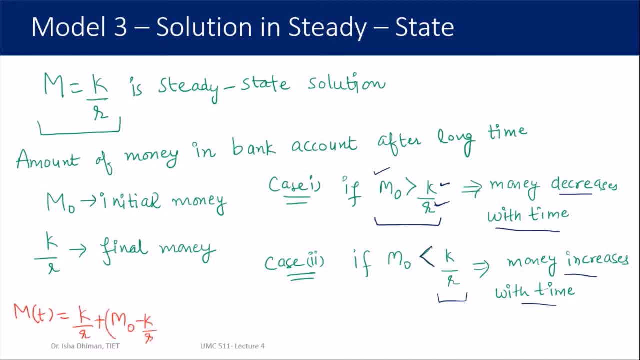 So this M T is K by R plus K by R, M naught minus K by R. this, this is a solution. I want to rewrite it in another way. this can also be written in this way: taking T naught is 0 again. that's just a simplification. putting. 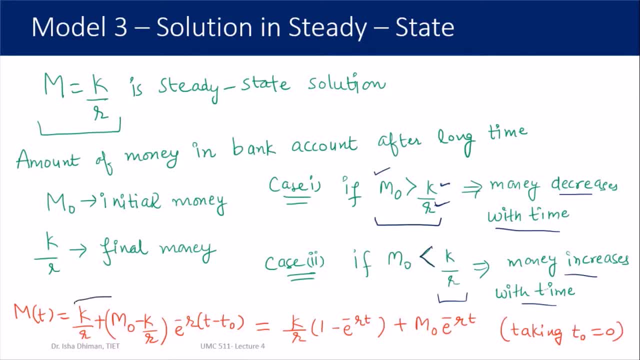 T naught equals to 0. I can rewrite this as this: so the same concept- this case 1 and case 2, is better understood from here, that if M naught is greater than K by R- you see carefully- at 1 minus E raised to power, minus RT, is going to be increasing with time. so if I'm not, is 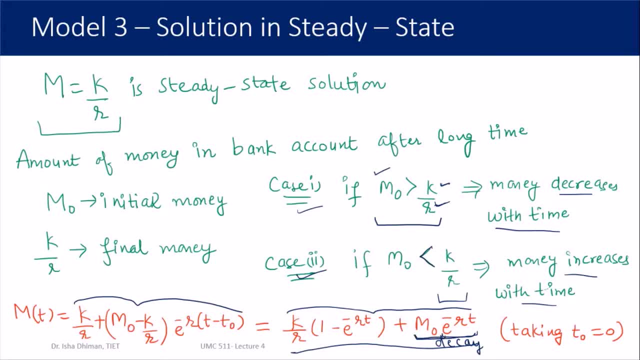 a positive factor. so if M naught is going to be large, so your money is eventually decreasing. and if E raised to power minus RT is decreasing with time, so 1 minus E raised to power minus RT is going to be increasing with time. so 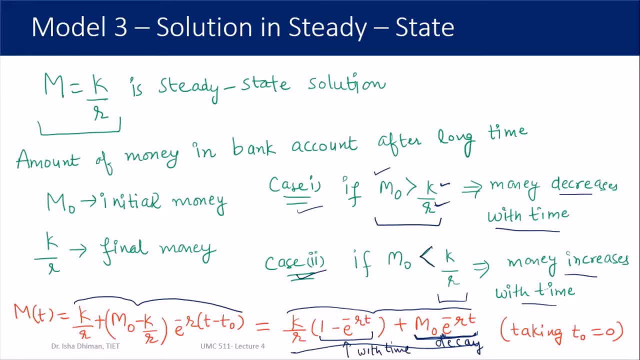 1. because it's just the opposite of that, because of a negative and subtracted from one. as time increases, this factor decreases, while this factor increases. so you can say the solution of this model consists of two parts: growth and decay. so if m naught is greater than k by r, so that means 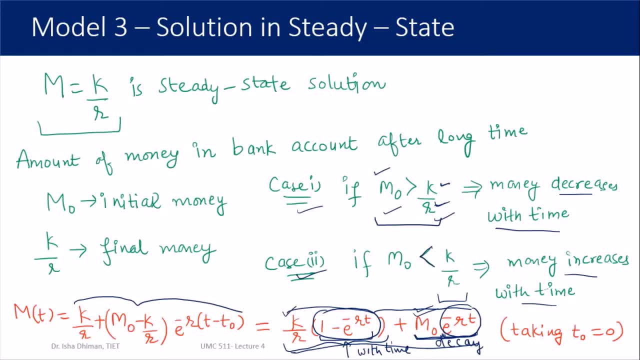 decay part coefficient is higher than the growth part, then your money is decreasing the time, while if the opposite happens, your money is increasing with time. so the interpretation which we got just by looking at the steady state solution, the same interpretation i can get from the solution. so 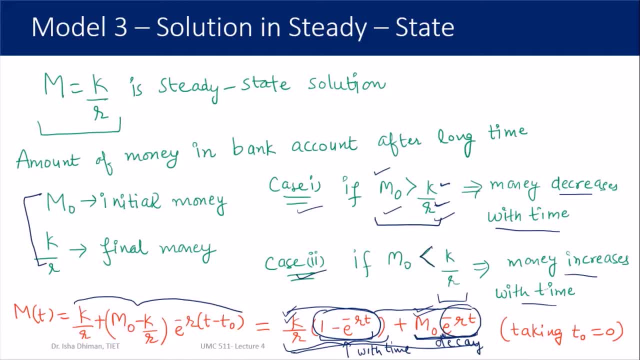 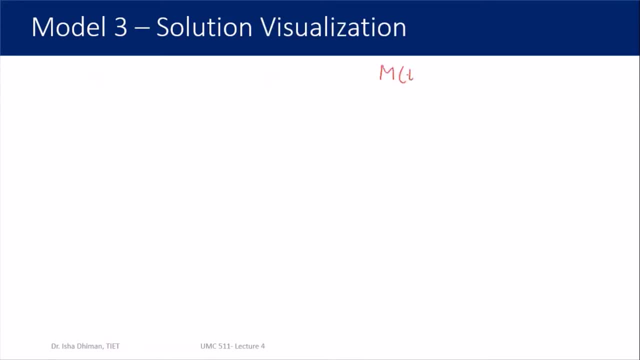 that's the physical or intuitive validation of the solution of model 3. so now let's visualize the same thing. so for different values of m? naught or k and r, i have plotted the solution curves and these are the graphs i'm getting. so i've fixed my m? naught equals to 10. and for different combinations of k and r. in fact i have 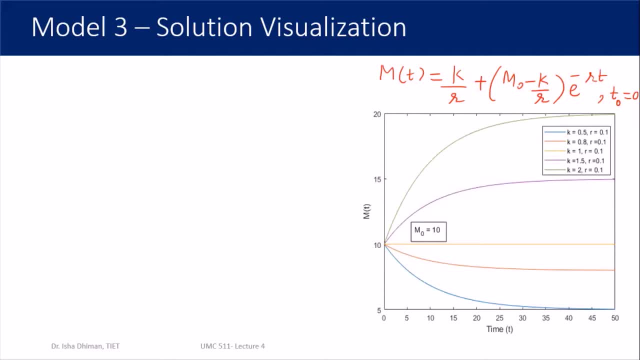 just varied k, while r i have kept at constant, at 0.1, and you can see from here that you see the blue curve first. so the blue curve is: k is 0.5, r is 0.1, so k by r is 0.5 by 0.1, which is 5, which